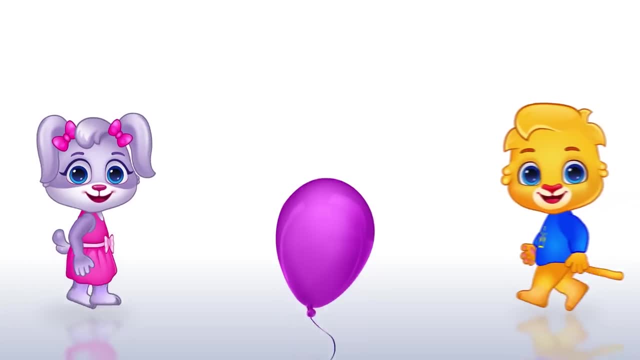 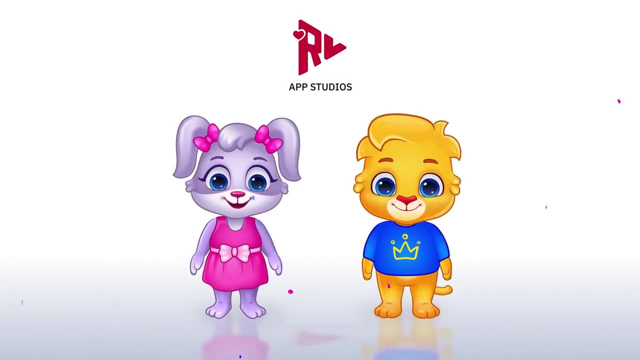 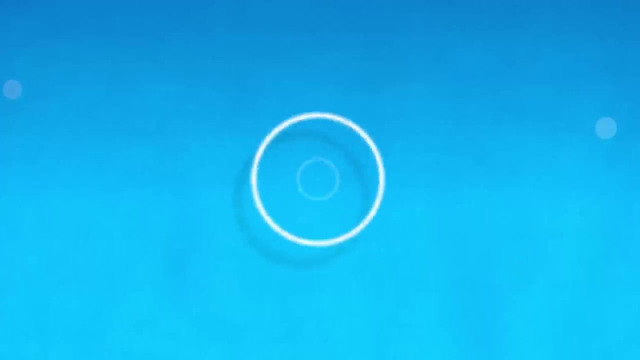 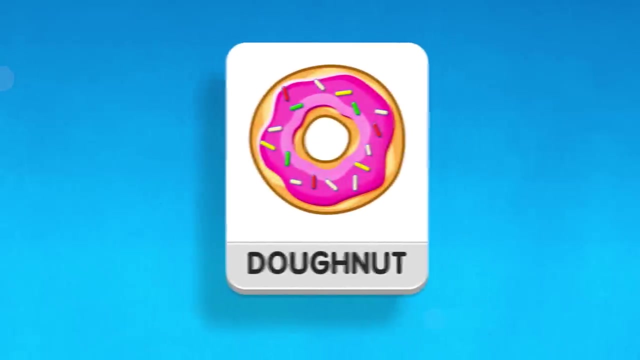 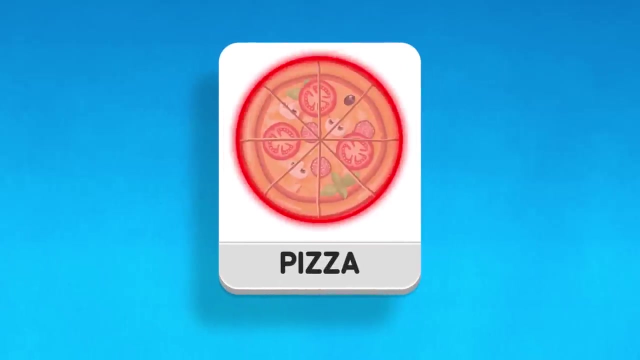 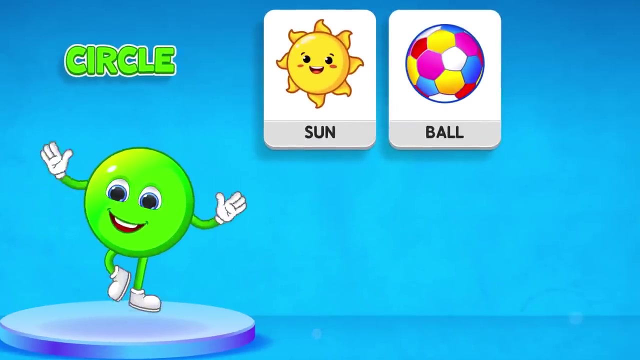 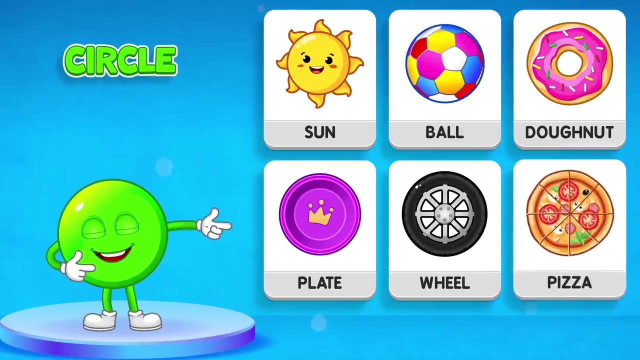 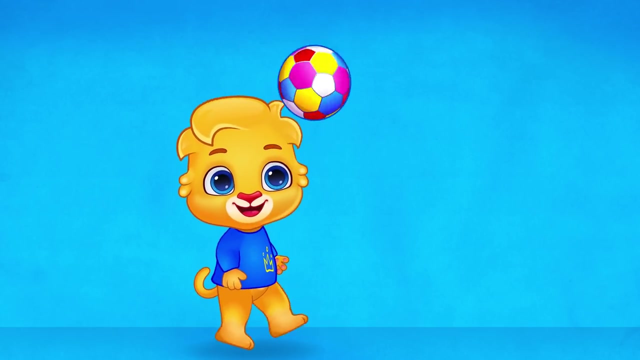 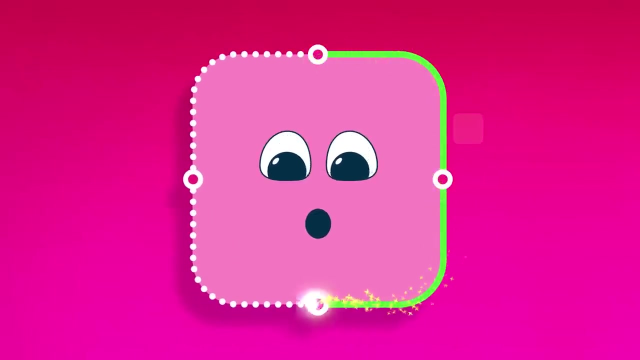 Hello, Oh Yeah, Circle, Circle, Circle Sun Circle Ball Circle Donut Circle Plate Circle Wheel Circle Pizza Circle. Hi, I'm Circle Sun Circle Ball Circle Donut Circle Plate, Circle Wheel Circle Pizza Circle. Ha ha ha, Square, Oh Square, Hi Square. 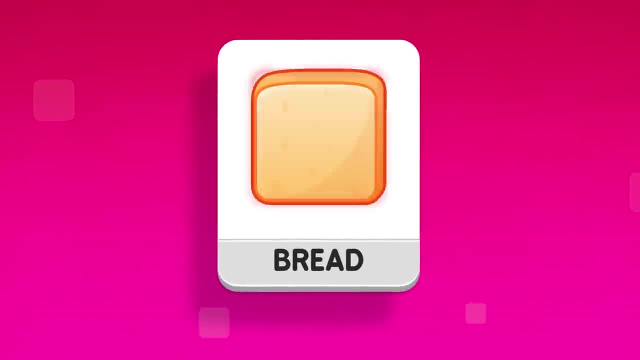 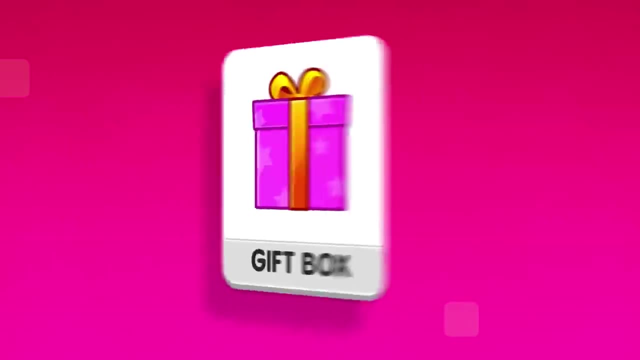 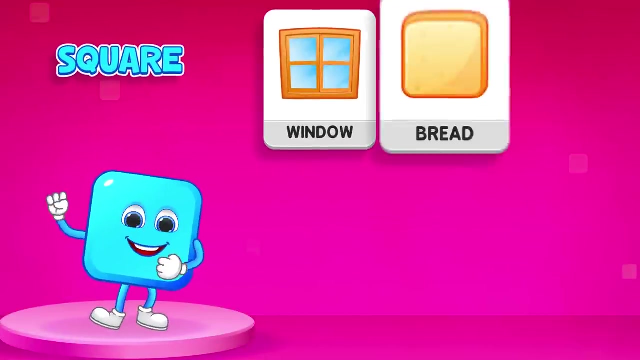 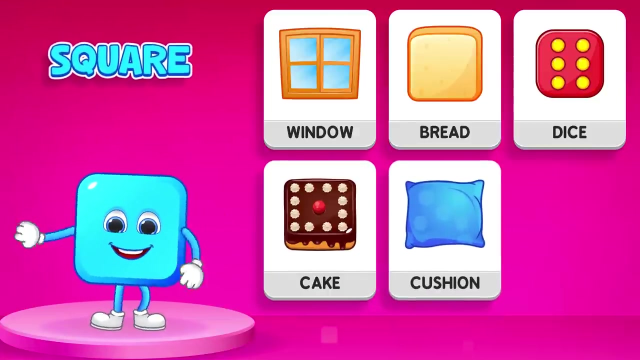 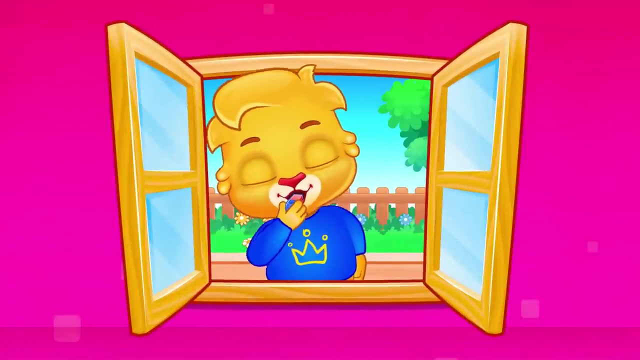 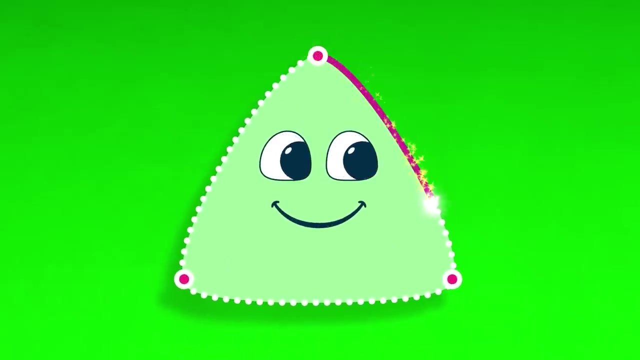 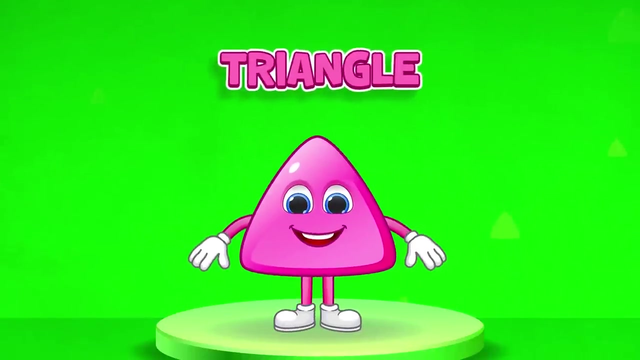 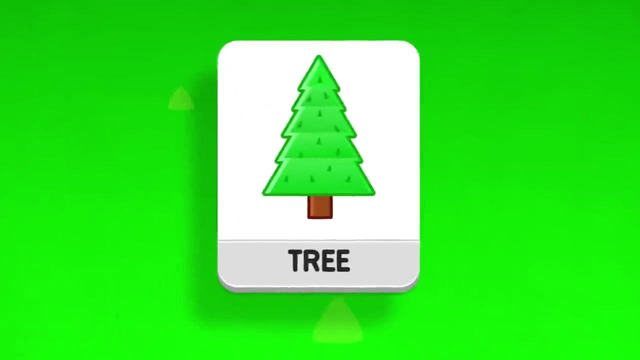 Window Square, Bread Square, Dice Square, Cake Square, Cushion Square, Gift Box Square. Hi, I'm Square Window Square, Bread Square, Dice Square, Cake Square, Cushion Square, Gift box Square. Triangle Triangle, Triangle, Cone Triangle, Sandwich Triangle, Cap Triangle, Tree Triangle. 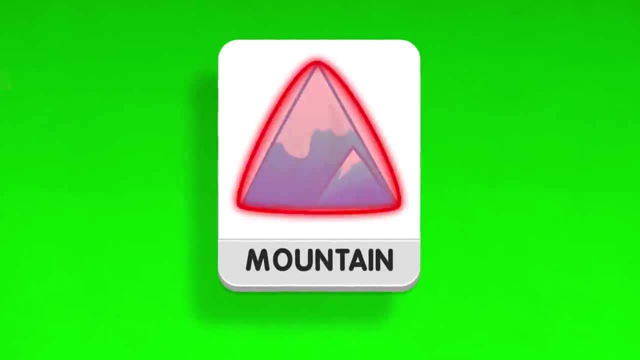 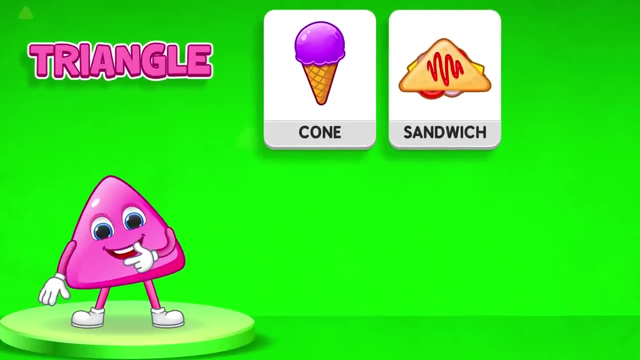 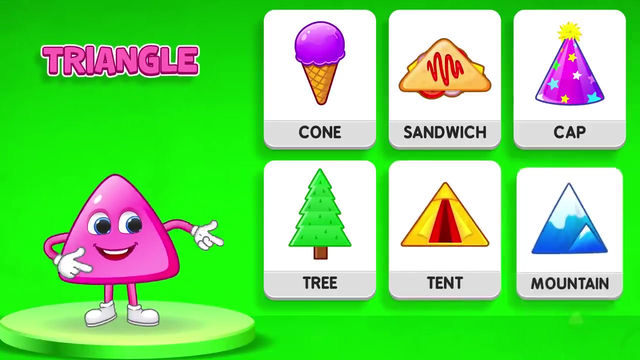 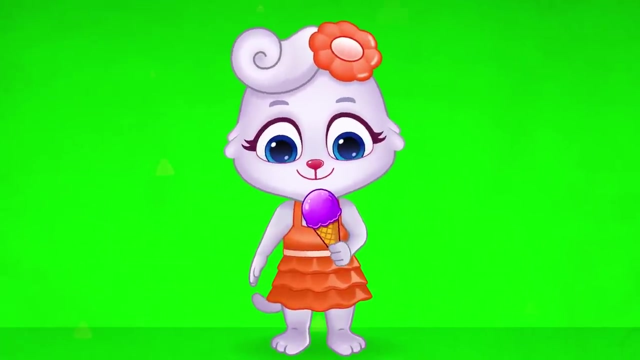 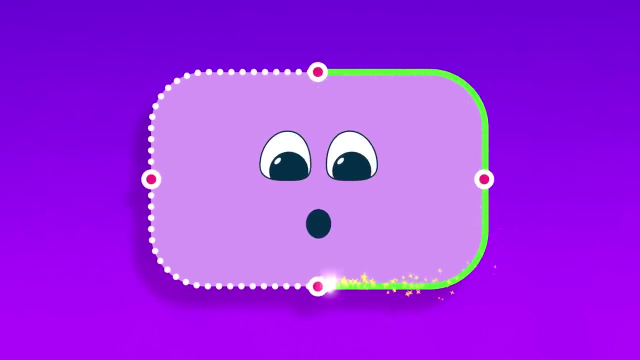 Tent Triangle Mountain, Triangle, Triangle. Hi, I'm Triangle Cone Triangle, Sandwich, Triangle, Cap Triangle, Tree Triangle, Tent Triangle Mountain, Triangle. Yay, Rectangle, Wow, Rectangle, Rectangle. 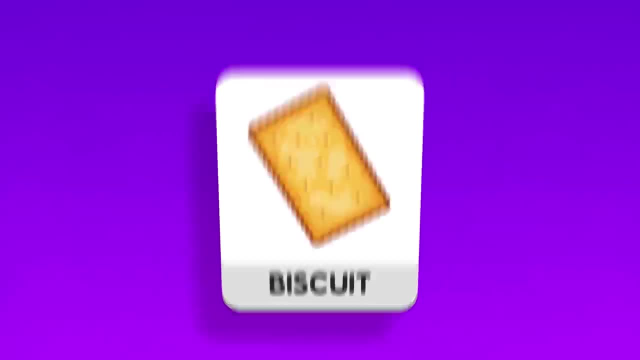 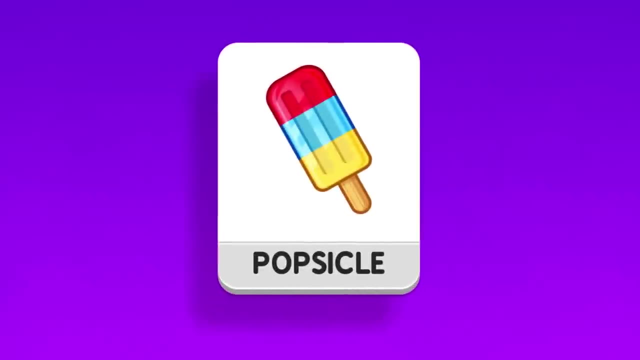 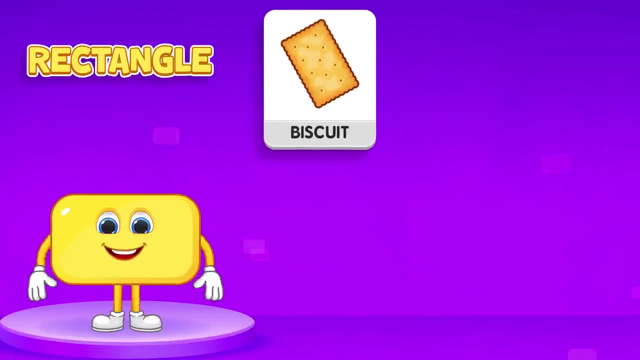 Hi. Rectangle Biscuit Rectangle Bag Rectangle, Television Rectangle. Door Rectangle Popsicle Rectangle Box Rectangle. Hi, I'm Rectangle Biscuit Rectangle Bag Rectangle, Television Rectangle. 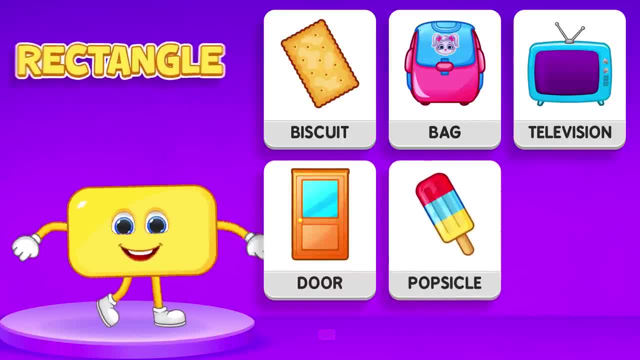 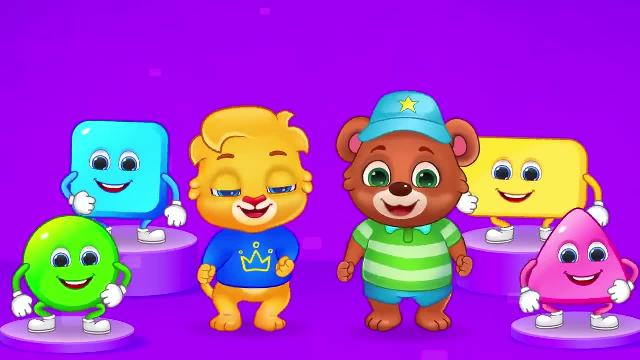 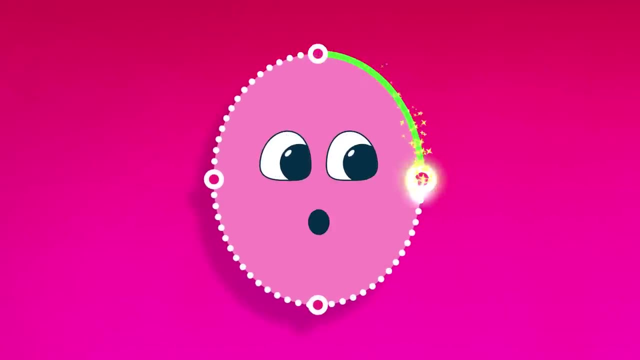 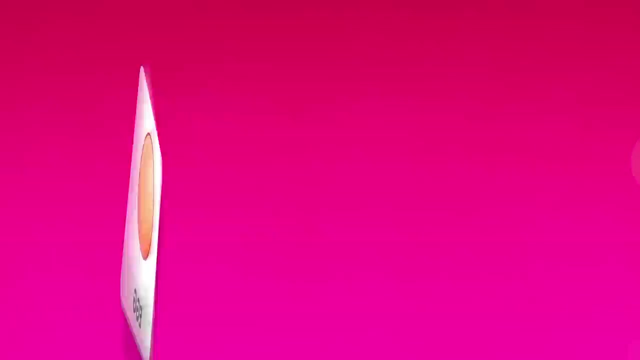 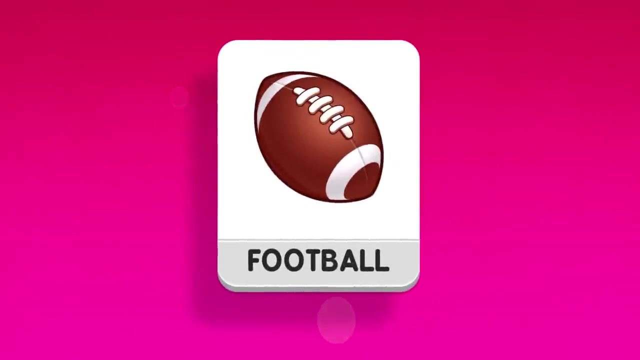 Door. Rectangle Popsicle, Rectangle Box, Rectangle Yay. Oval Whoa. Oval Hi. Oval Egg. Oval Grapes. Oval Watermelon. Oval Football. Oval Mirror. Oval Pineapple. 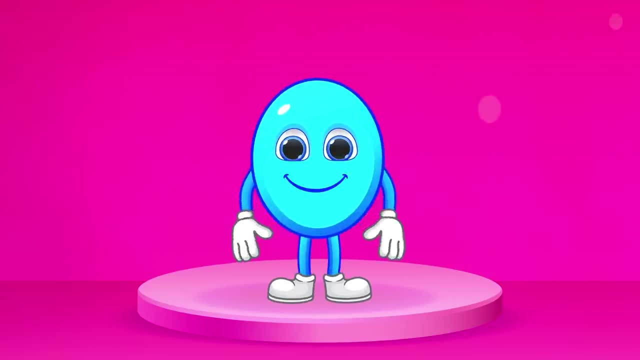 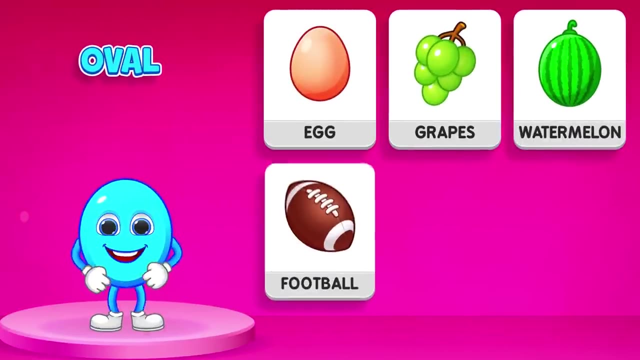 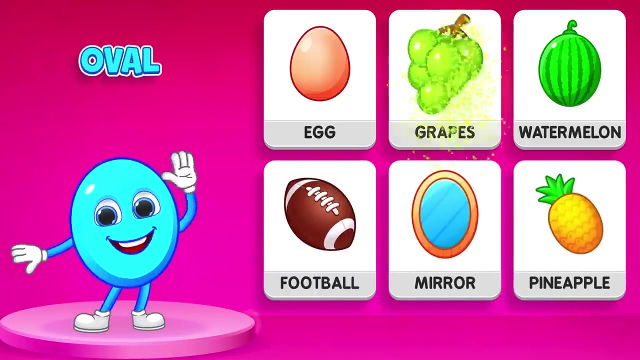 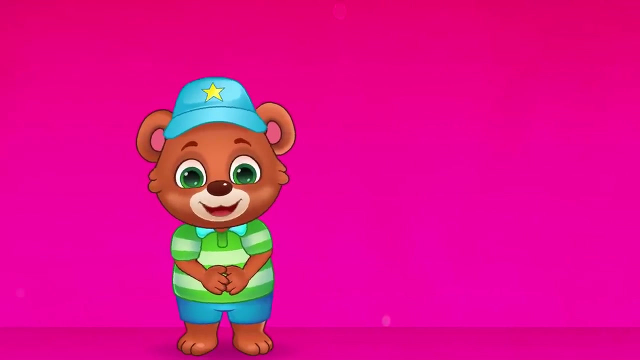 Oval- Hi, I'm. Oval Egg. Oval Grapes. Oval Watermelon. Oval Football. Oval Mirror. Oval Pineapple, Oval Yay, Mmm, Hahaha, Hahaha, Rhombus. 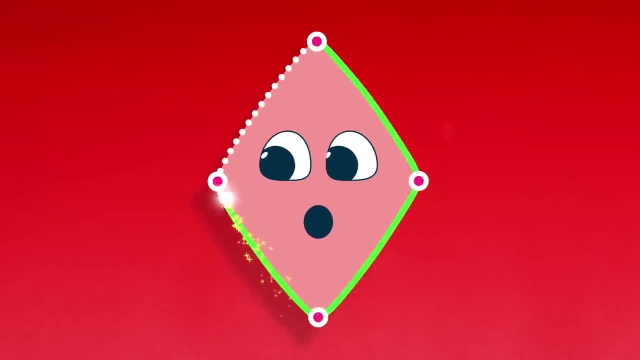 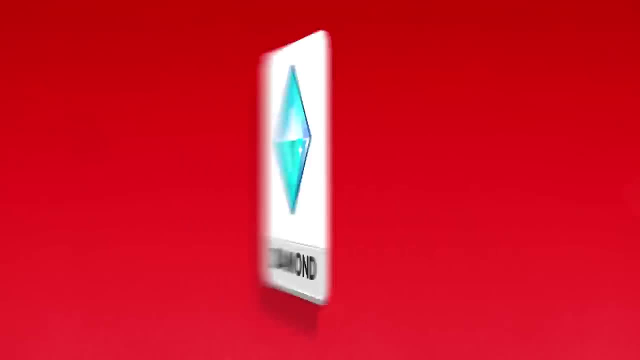 Whoa Rhombus, Rhombus, Rhombus Rhombus Rhombus, fish Rhombus, Diamond Rhombus Rhombus, Kite Rhombus, Toy Rhombus. 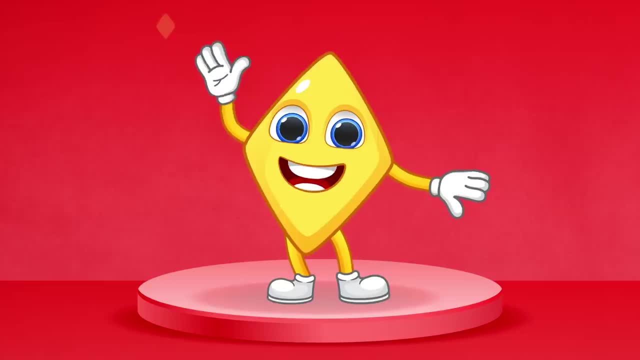 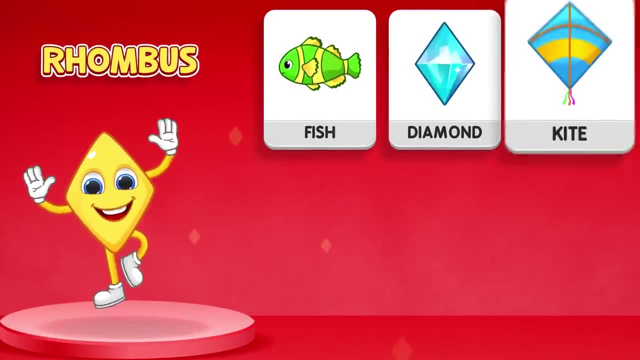 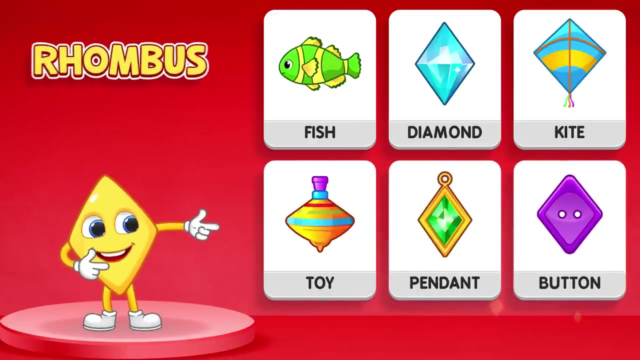 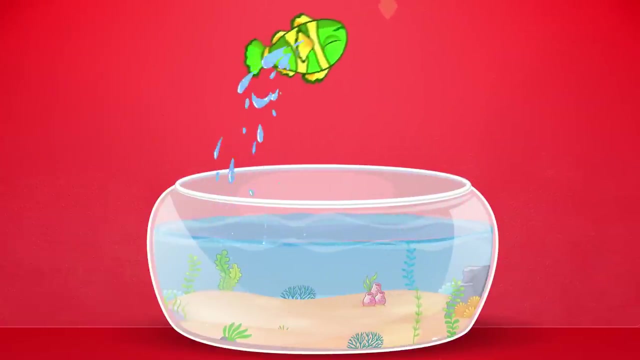 Fatten Rhombus Button Rhombus. Hi, I'm rhombus Fish, Rhombus Diamond Rhombus Kite Rhombus Button Rhombus, Semicircle, Oh. 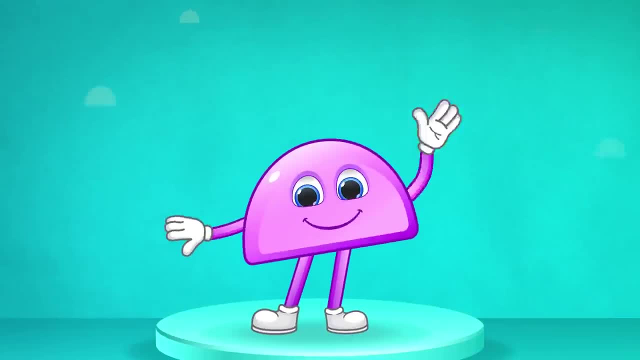 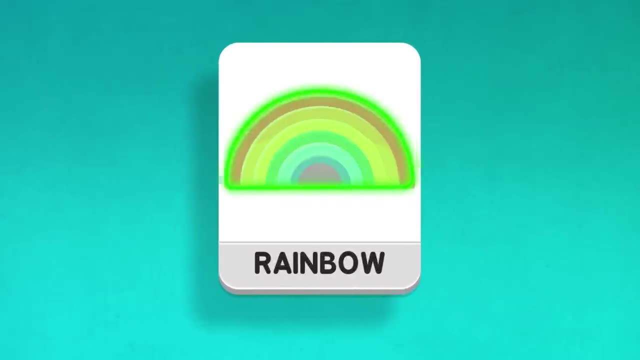 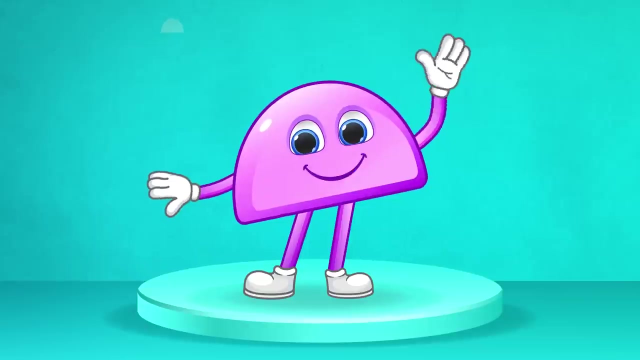 Semicircle Hi. Semicircle Umbrella. Semicircle Igloo Semicircle, Rainbow Semicircle, Mushroom Semicircle, Cup. Semicircle, Cap Semicircle. Hi, I'm Semicircle. 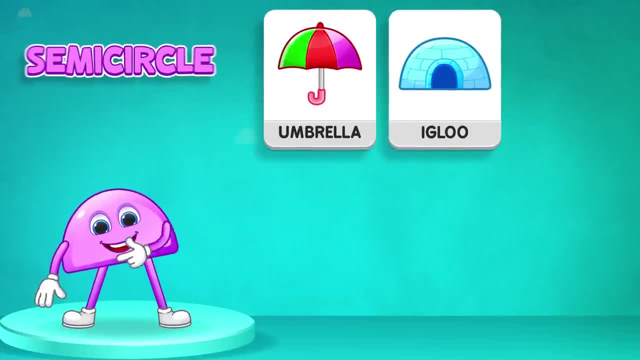 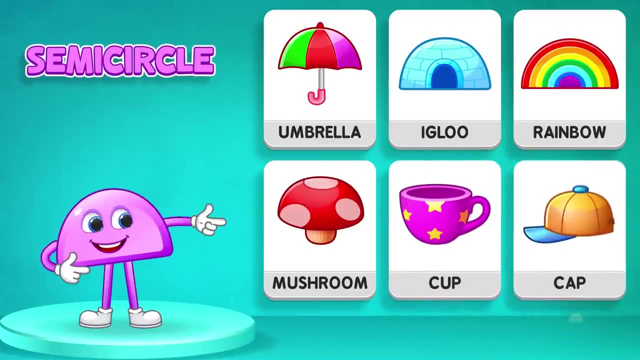 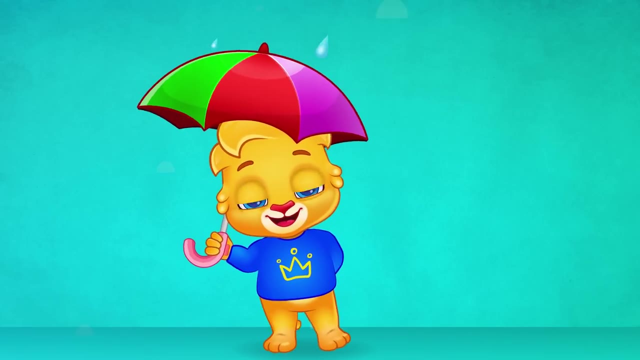 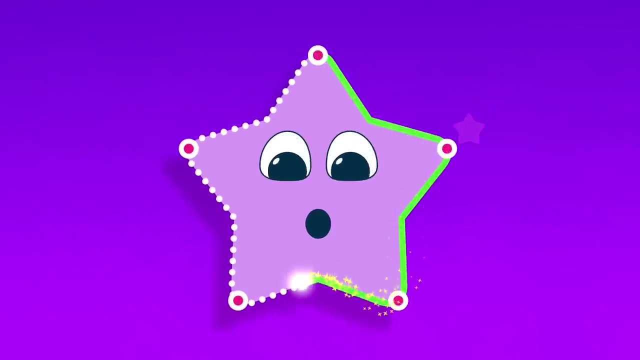 Umbrella, Semicircle, Igloo Semicircle Rainbow Semicircle, Mushroom Semicircle, Cup Semicircle, Cap Semicircle. Yeah, Star, Oh Star, Hi Star, Starfruit. 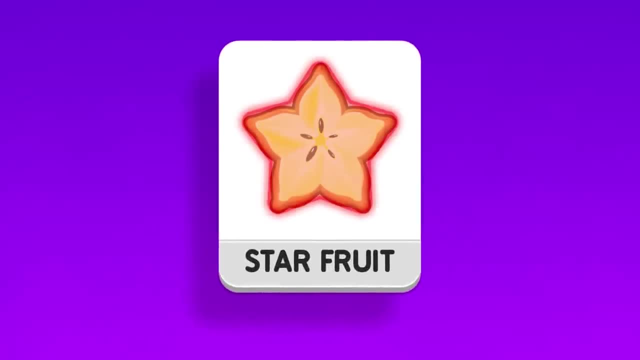 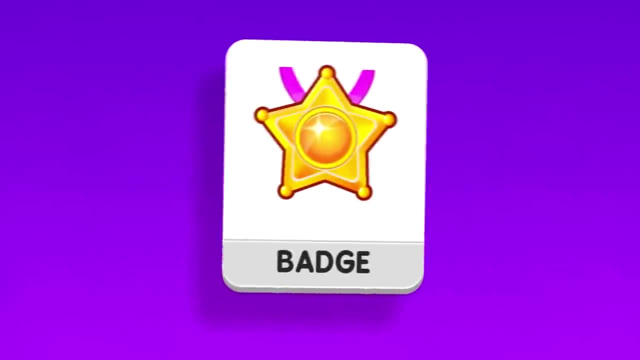 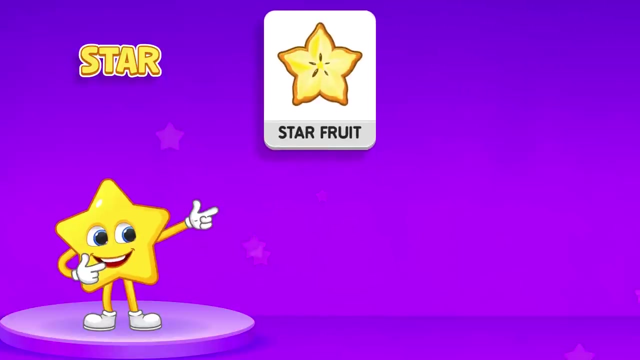 Star Starfish, Star Ring Star Balloon Star Badge. Star Cookies Star. Hi, I'm Star Starfruit. Star Starfish, Star Ring Star Balloon Star Badge. 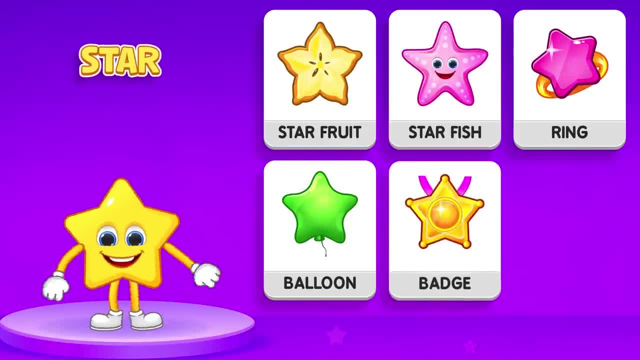 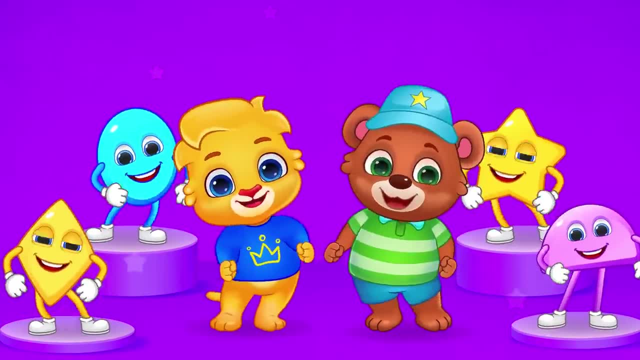 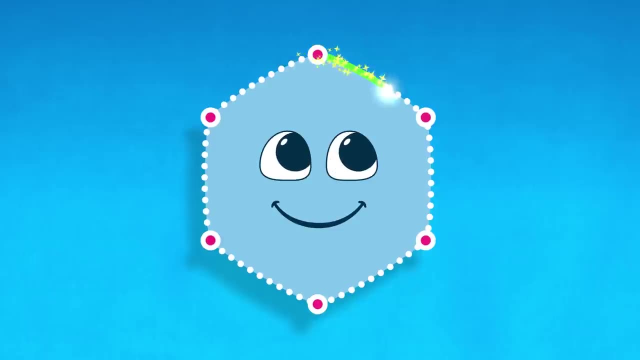 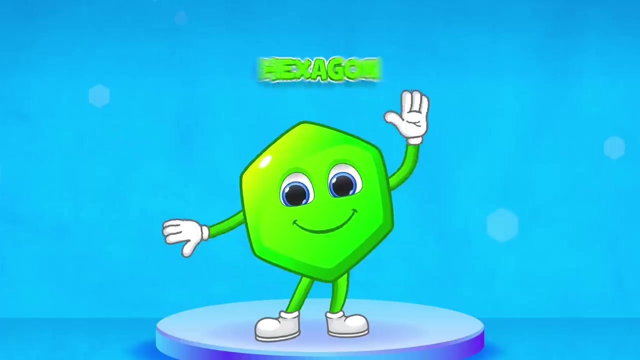 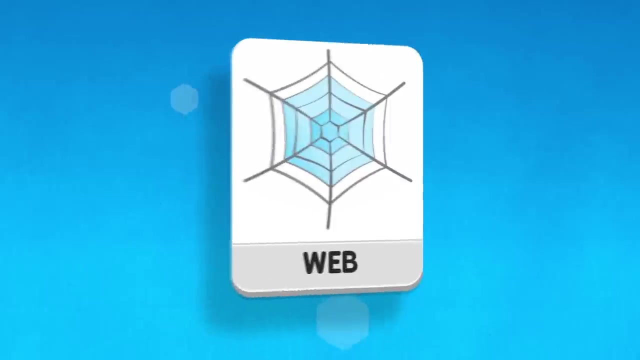 Star Star, Star Badge, Star Cookies, Star. Hexagon, Oh, Hexagon Hi. Hexagon Honeycomb. Hexagon Nut, Hexagon Snowflake, Hexagon Web, Hexagon Metal. 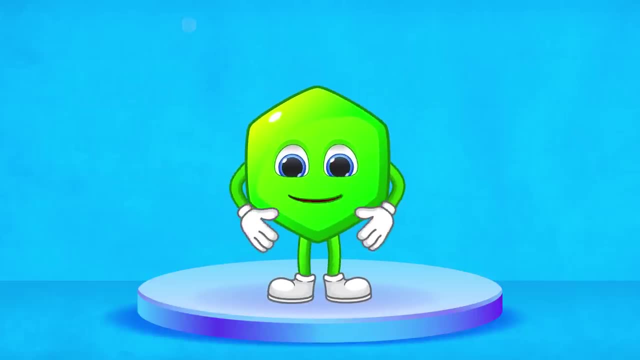 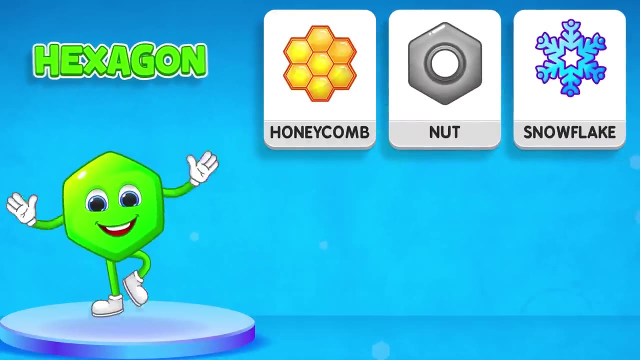 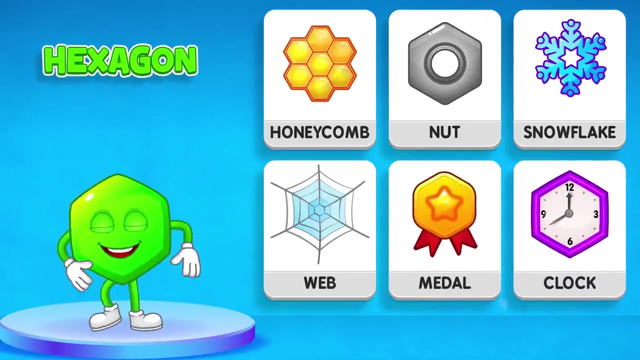 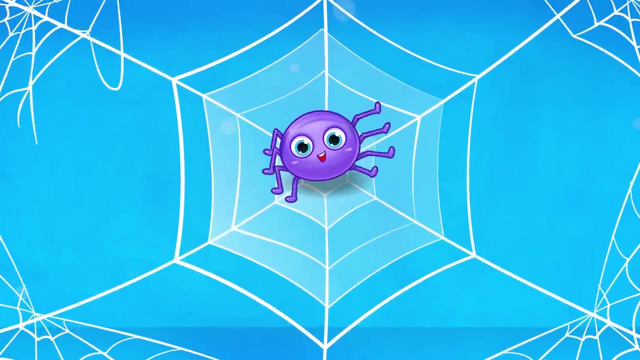 Hexagon Clock- Hexagon. Hi, I'm Hexagon Honeycomb, Hexagon Nut. Hexagon Snowflake. Hexagon Web. Hexagon Metal. Hexagon Clock- Hexagon, Hexagon, Hexagon. 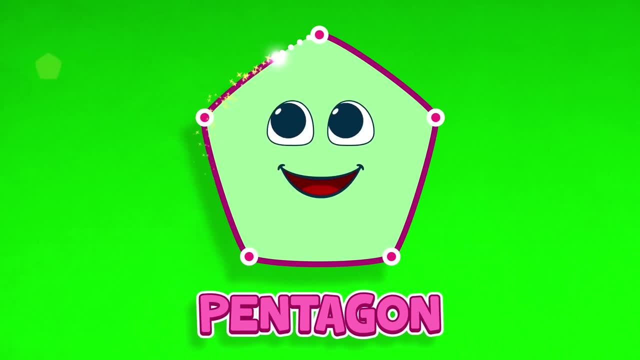 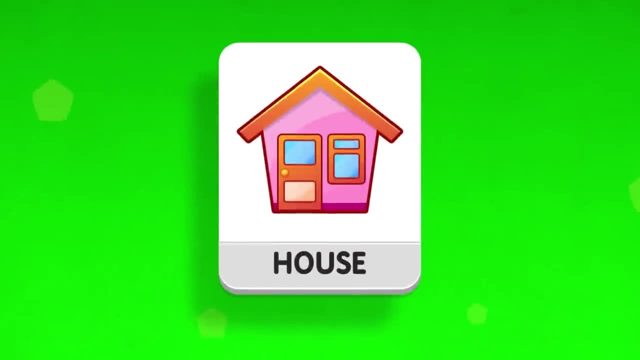 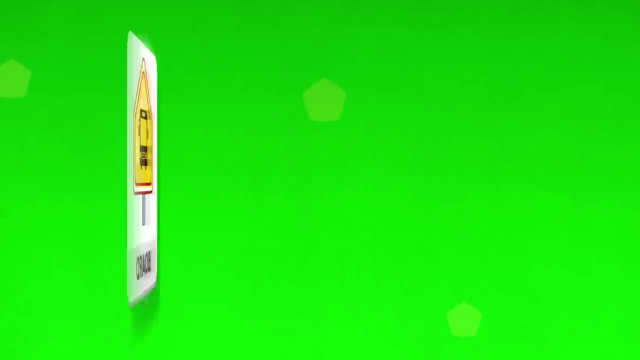 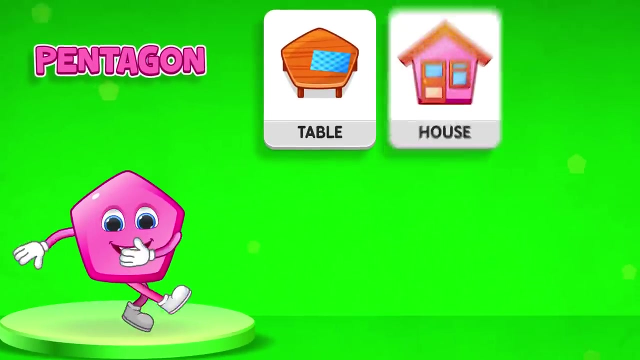 Hexagon, Oh, Hexagon, Hexagon, Hexagon Table, Hexagon House, Hexagon Earrings, Hexagon Envelope, Hexagon Hut, Hexagon, Pentagon hut. I'm Pentagon table, Pentagon house, Pentagon earrings, Pentagon envelope. 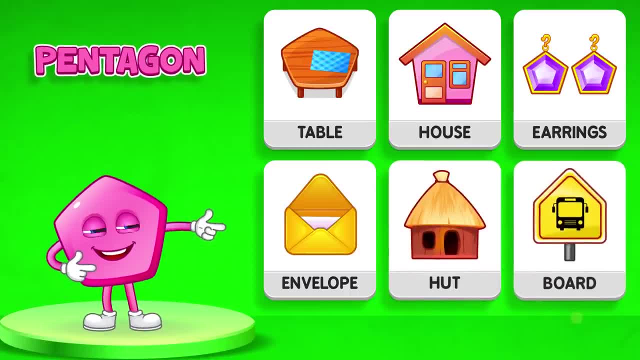 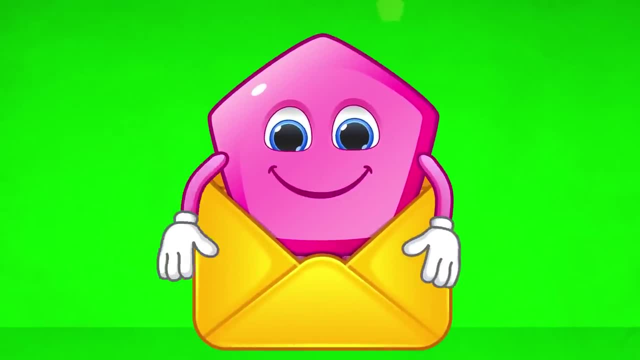 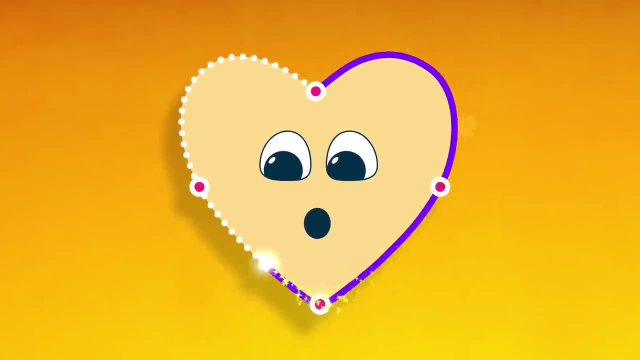 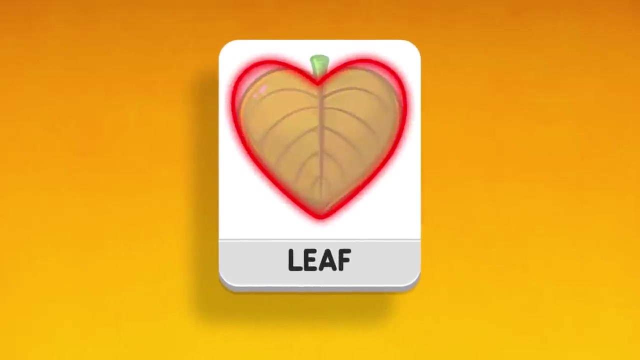 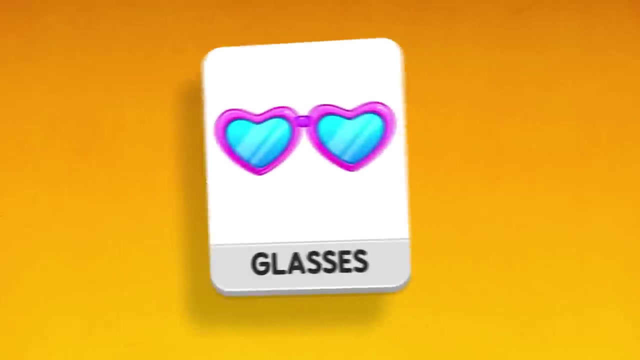 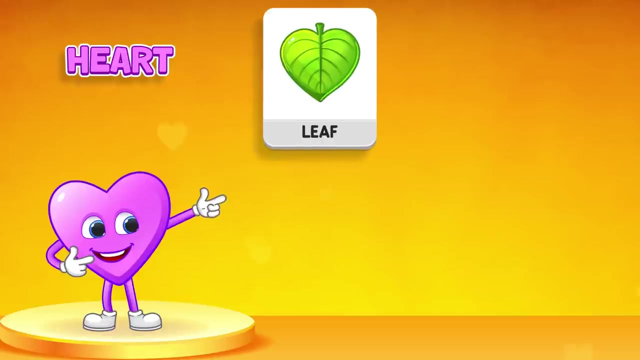 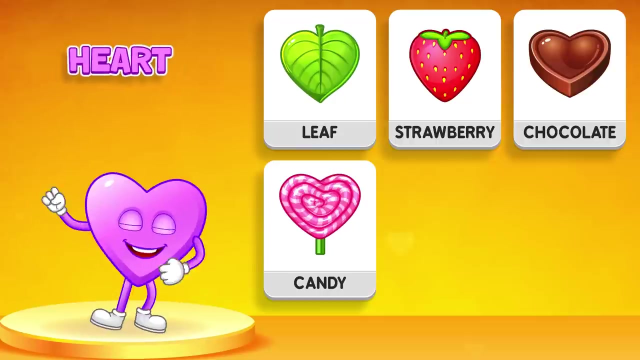 Pentagon hut, Pentagon Ford, Pentagon Heart, heart, heart leaf heart, strawberry heart, chocolate heart, candy heart glasses. heart cupcake, heart, Heart hut. I'm heart leaf heart, strawberry heart, chocolate heart, candy heart glasses. 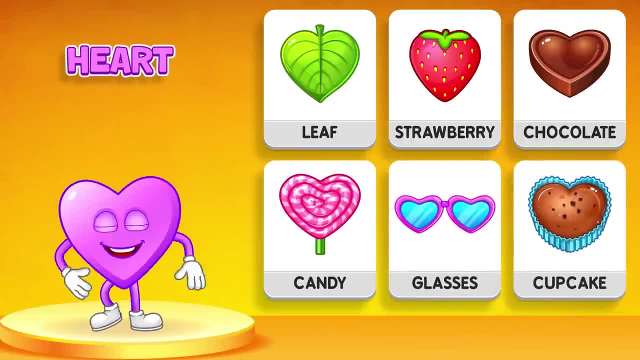 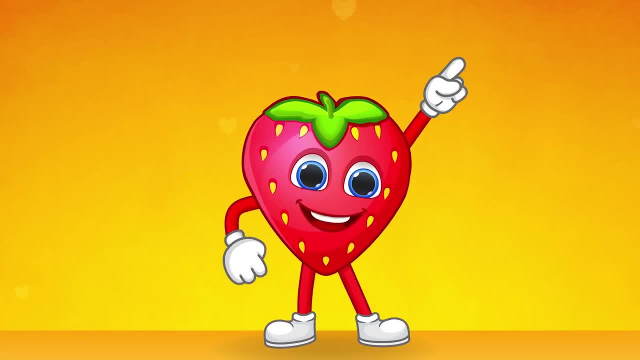 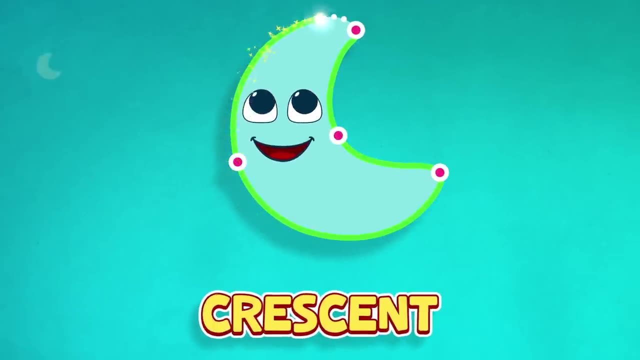 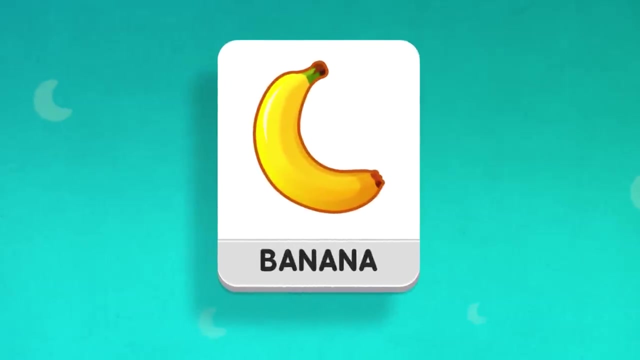 heart cupcake heart. Yay. Uh-huh, Yeehaw, Uh-huh. Crescent, Oh. Crescent Crescent, Crescent. Crescent Banana. Crescent Moon, Crescent Cashew, Crescent Red chili. Crescent Brinjal Crescent Hi I'm Crescent. Crescent Crescent Banana. Crescent Moon. Crescent Cashew. Crescent Red chili Crescent Brinjal Crescent Crescent Banana Crescent- Blu-ray. 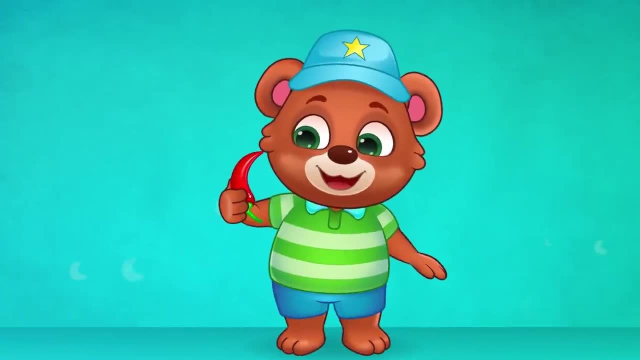 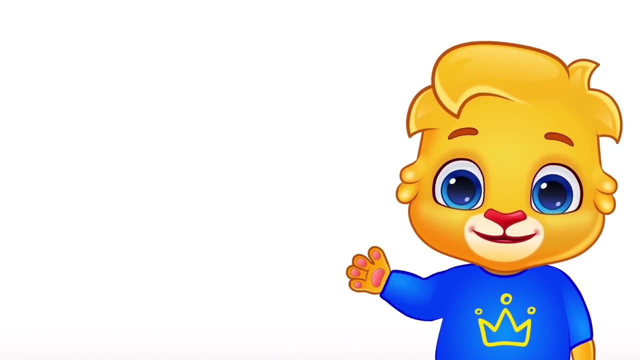 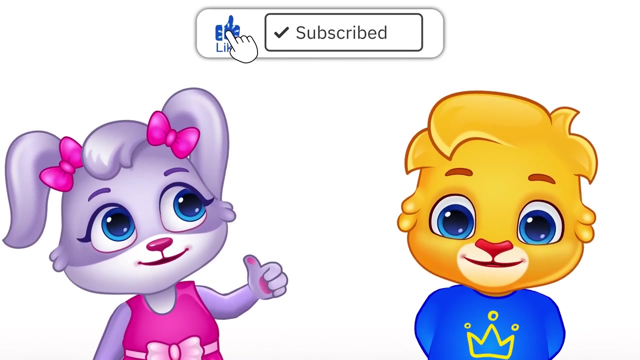 Crescent Green, Slipper Green Green. Yeah, Ah ha, ha ha. Hey kiddos and parents, hope you enjoyed the video. Can you subscribe to our channel and hit that like button? It really, really, really helps to recommend our video to other parents on YouTube. 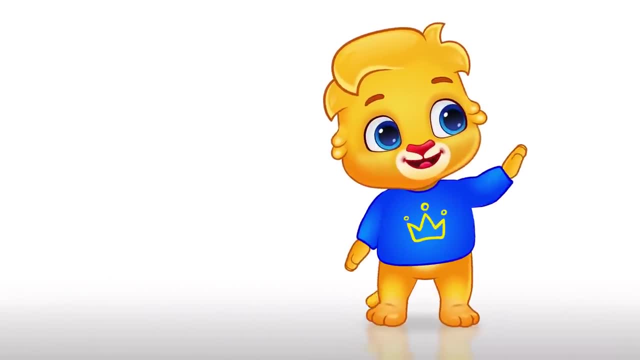 Bye. bye, Hey, Ruby, Wait for me. Bye-bye, It's gift time. 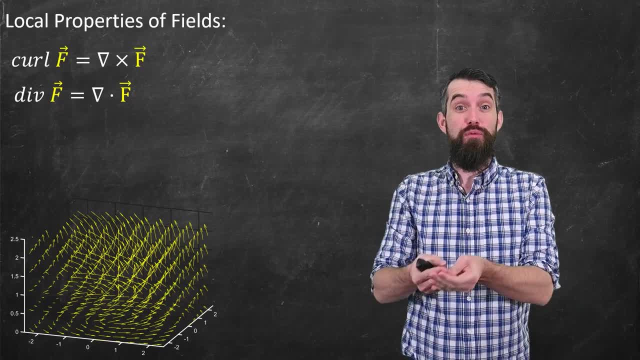 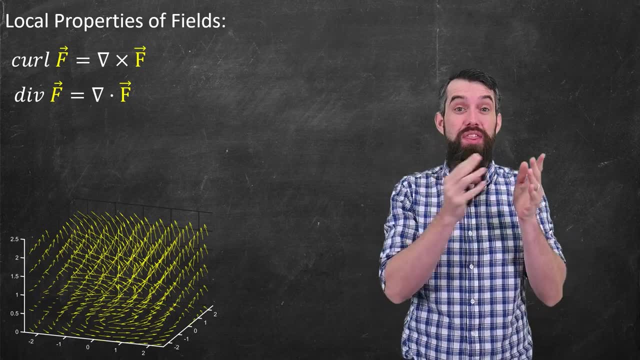 In this video we're going to walk through the major theorems of vector calculus, Green theorem, Stokes' theorem and divergent theorem And we're going to see that all of these theorems have a common theme that can be unified with an underlying principle And indeed, 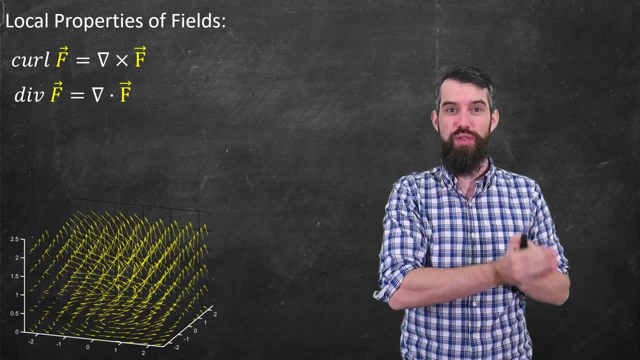 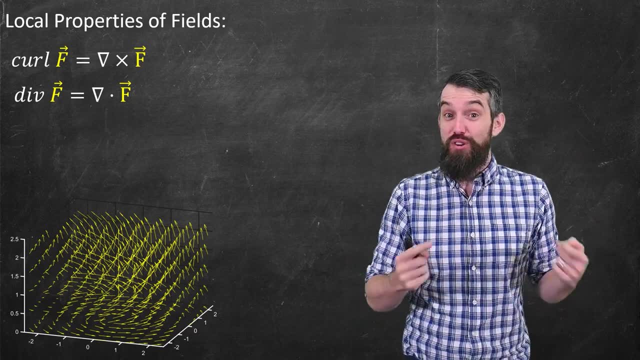 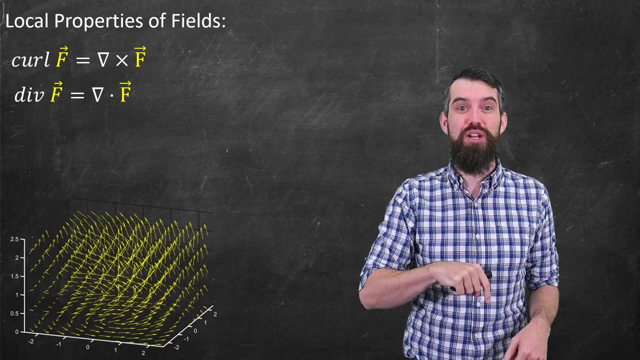 a theme that extends all the way back to the fundamental theorem of calculus. Now, this video is actually the final video in my vector calculus playlist. If you've been following along since the beginning, well, congratulations, you are now done. And if you're just finding the video right now, well, down in the description I have the entire playlist. 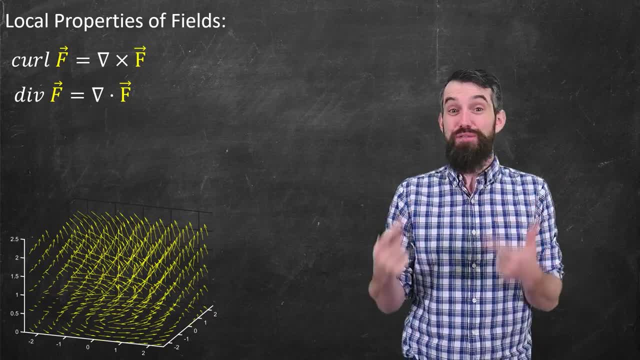 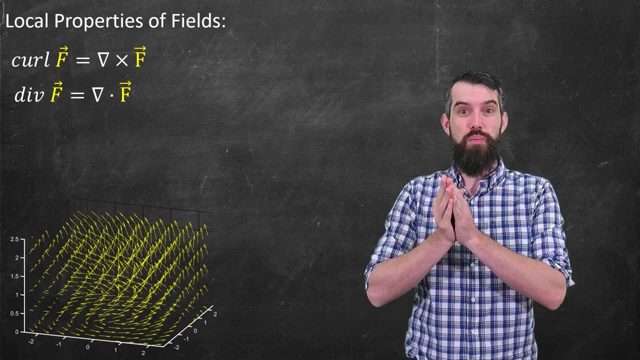 so you can go back and see all the different concepts we've talked about, And so this video was really meant as a summary of some of the themes we've talked about and putting it all together, hopefully, in one major picture. So the first thing to talk about, if I have a vector field,